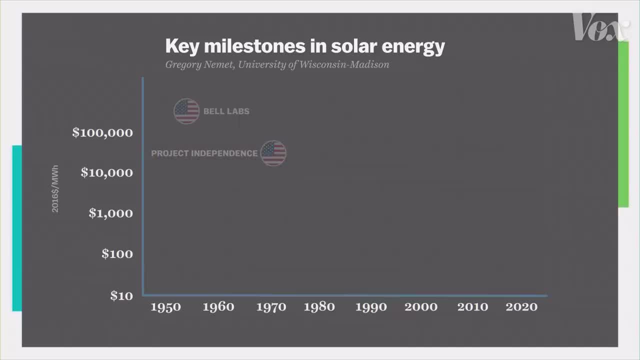 President Reagan canceled Project Independence. Fortunately, two countries were ready to step in and put Maycock's hypothesis to the test. Like the US, Japan had been hit hard by the oil crisis in the 70s. They started funding solar research and development around the same time. 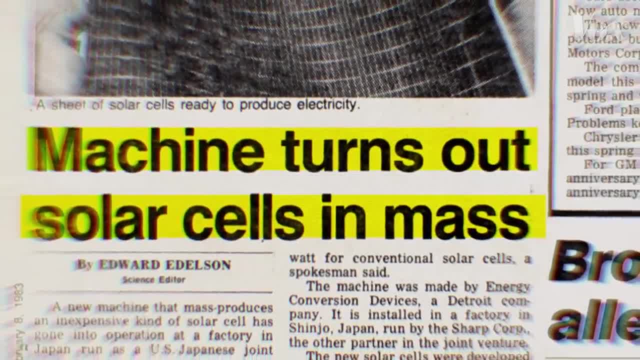 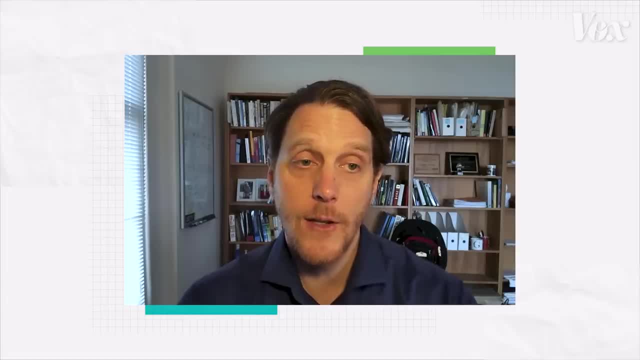 And soon they developed solar cells small and powerful enough to run watches, calculators and toys- Trivial in terms of the growth And in terms of the global energy system, But crucial in that large companies were now becoming interested in solar. 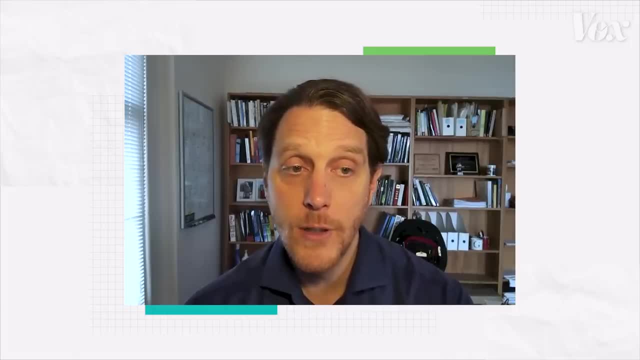 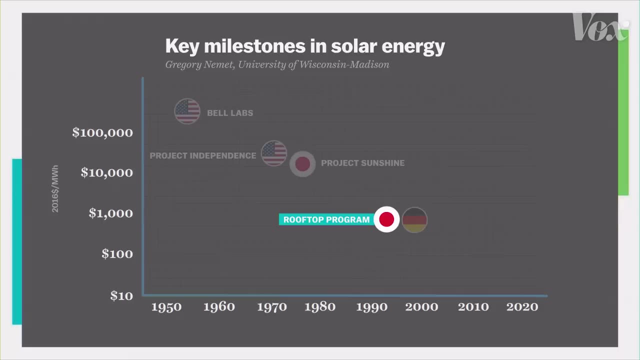 And, crucially, figuring out how to construct solar at really low- low cost. That know-how came in handy when the Japanese government announced a major subsidy for rooftop solar in the mid-90s, But the global market for solar technology was still relatively small. 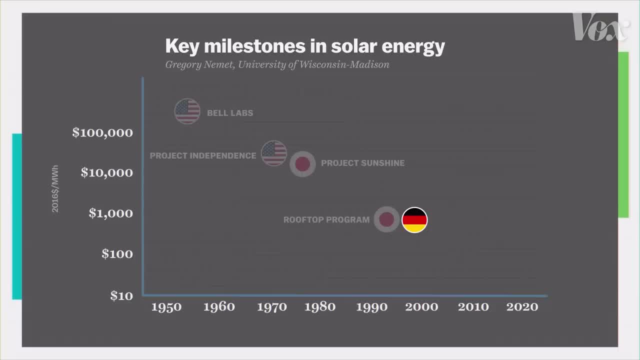 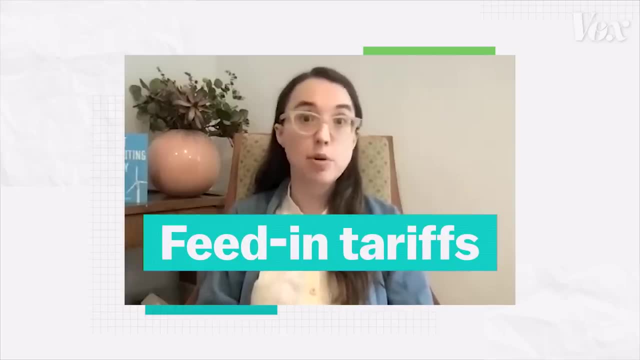 Until Germany stepped in and truly changed the game, The most important policy on this whole chain. if I had to pick one, it would be the German feed-in tariff. Feed-in tariffs, which was basically a program that deployed solar at scale. Here's how it worked. 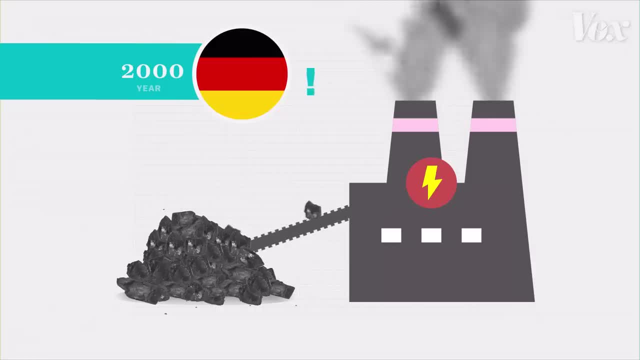 Starting in 2000,. the German government basically said to power companies: hey, if you can start producing renewable energy, we will buy it from you, We promise For double the market price, And we will keep paying you at that rate for the next 20 years. 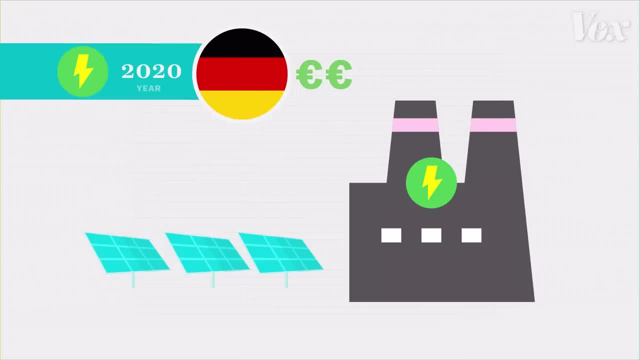 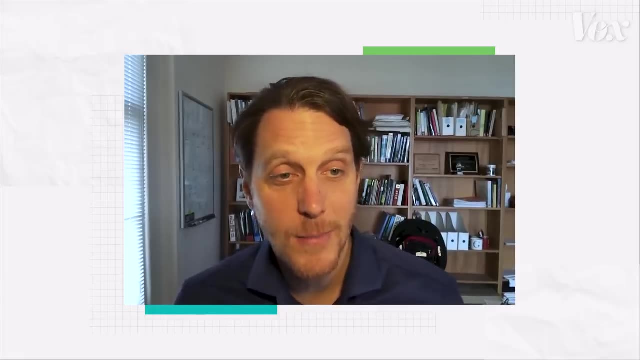 And so for developers of solar projects in Germany, all of a sudden, it became a no-brainer to do this, Even though Germany is not the sunniest place in the world, Companies responded to the incentives by building solar farms like this one. 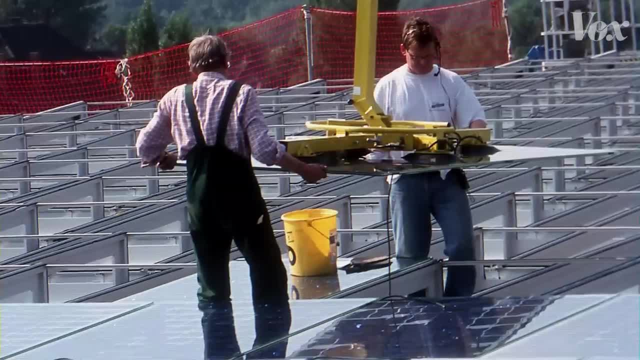 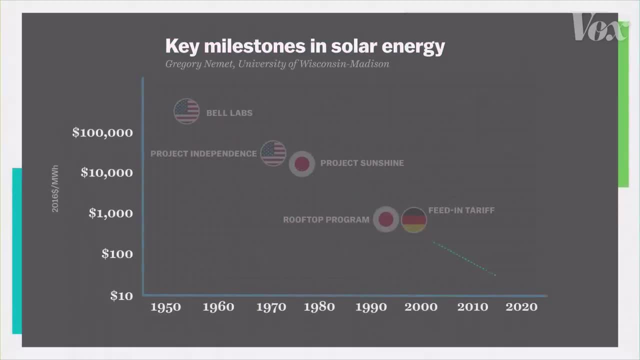 In one year the installations for solar went up by a factor of four, and then it just grew. The more panels they produced, the cheaper it got to generate electricity with solar. Then another country picked up the baton and made solar cheaper than even Maycock could have imagined. 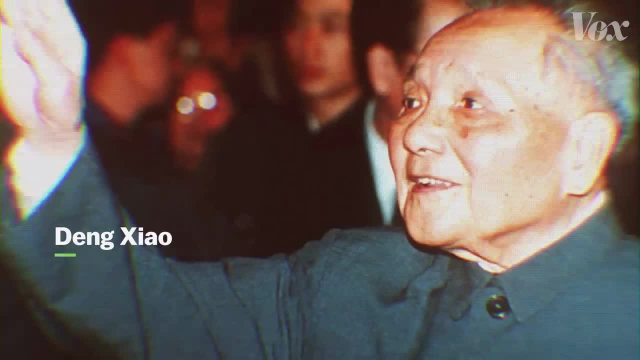 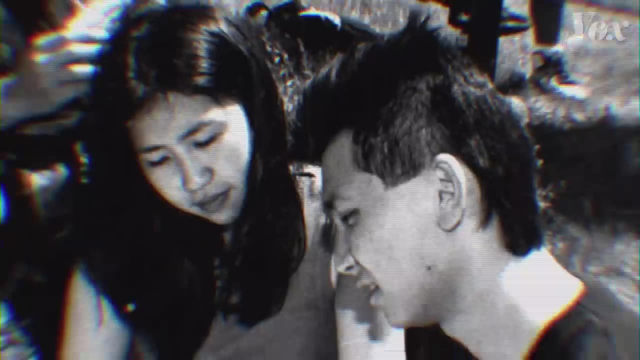 So it really starts with Deng Xiaoping in the 1980s and had this plan for a thousand Chinese students To go abroad and come back and see what they came back with. One group of students went to the University of New South Wales in Australia. 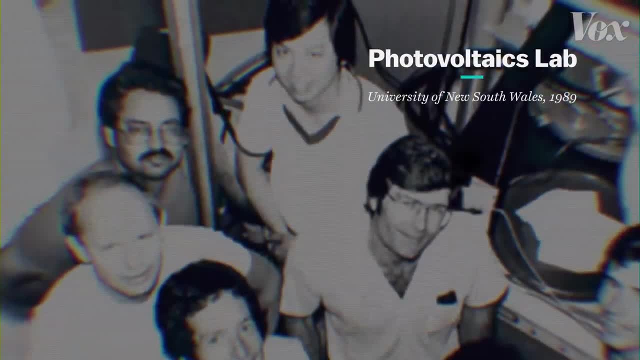 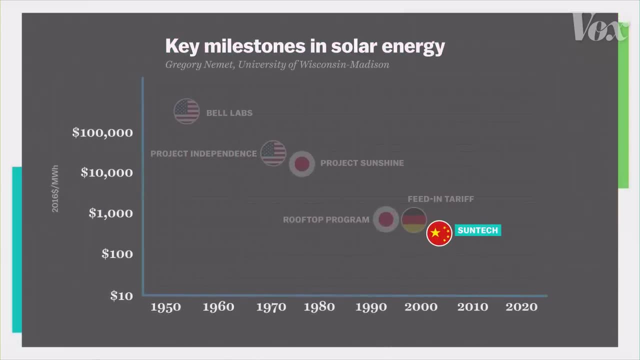 where they worked with a team that was producing some of the most efficient solar cells in the world. After a few years, one of those students went back to China and opened up the country's first commercial solar manufacturer, SunTech, in 2002.. 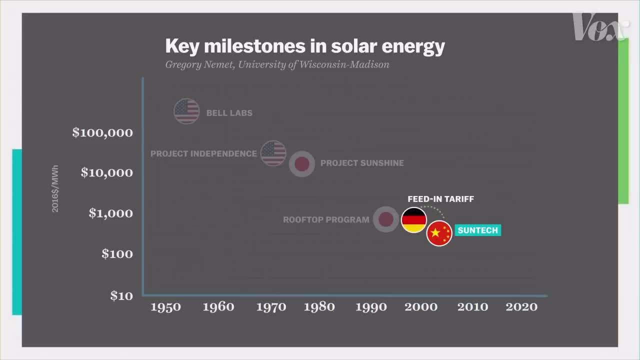 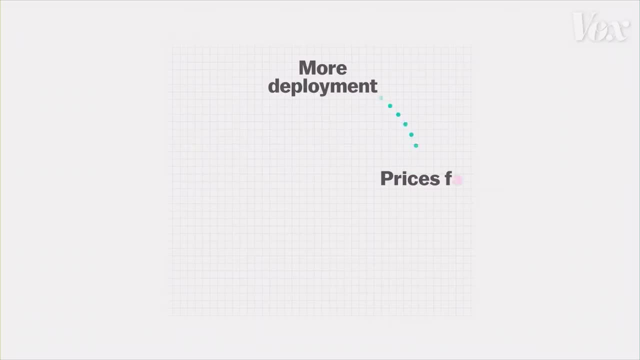 With that new German law in place, the company had so much success selling solar panels to Germany. SunTech's success attracted competitors, which helped drive down prices, In part because all of this demand inspired Chinese manufacturers to produce at an unprecedented scale. Policymakers around the world noticed the falling prices and wrote laws to create. 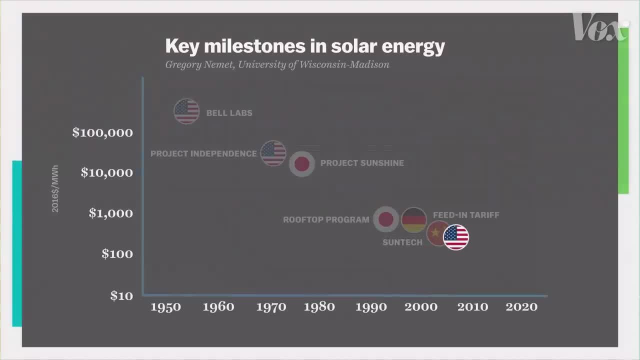 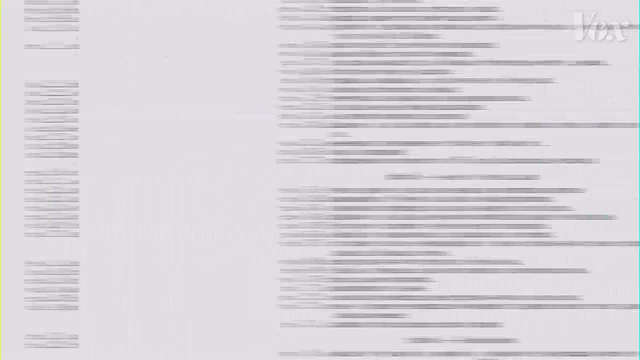 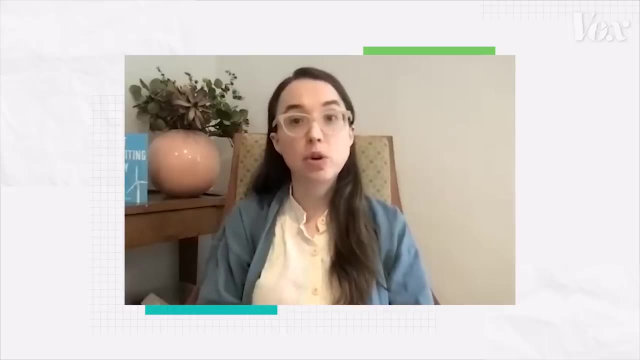 new markets in their countries, including the United States. The United States passed an important law. It's called the Energy Policy Act of 2005.. And buried deep within that law was an investment tax credit. Sounds kind of boring, but it turns out it was absolutely critical to deploying solar, because what it said was that it 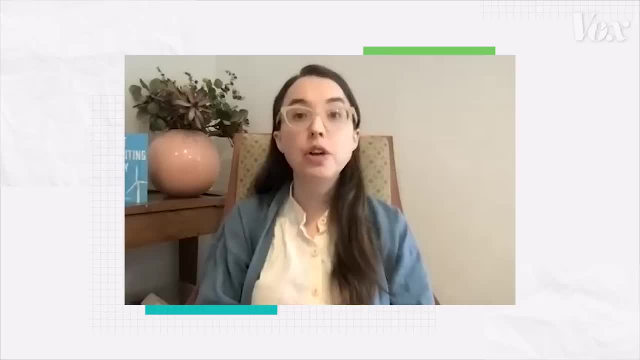 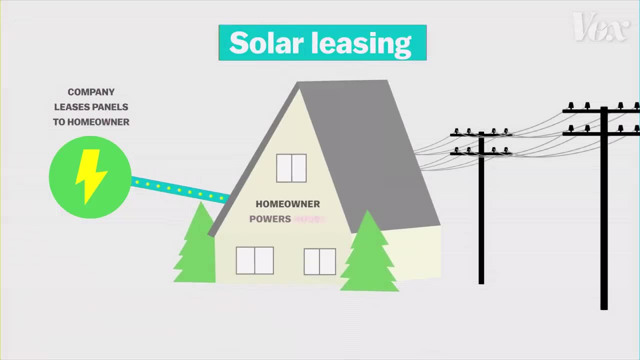 meant that if you put out a new solar project, you can get 30 percent of those costs back through a tax credit. This sparked a phenomenon called solar leasing, where companies would look for places to put solar so that they could reduce the amount they owed the federal government in. 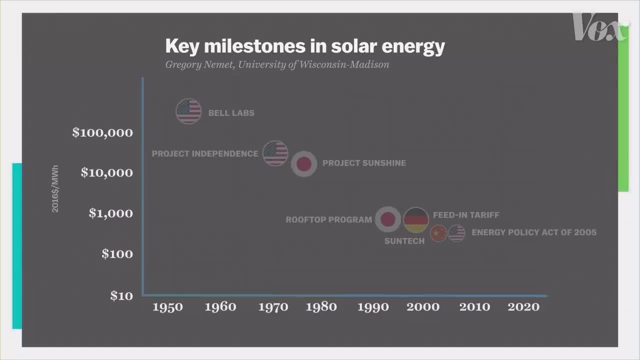 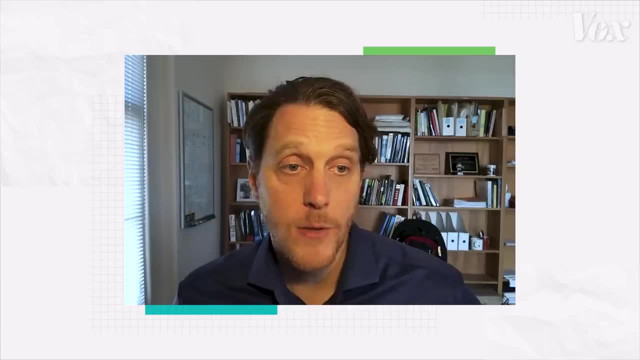 taxes. Other policies helped create markets for solar modules in Spain, Italy and, crucially, in China. The Chinese devised their own subsidy program that was modeled on the German one, where you get a guaranteed price. By 2011,, China was not only going to have to pay for solar, but 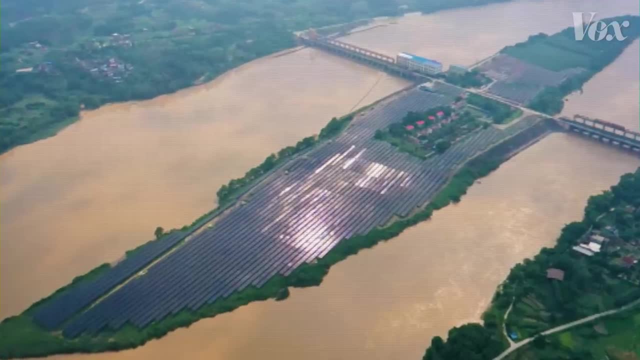 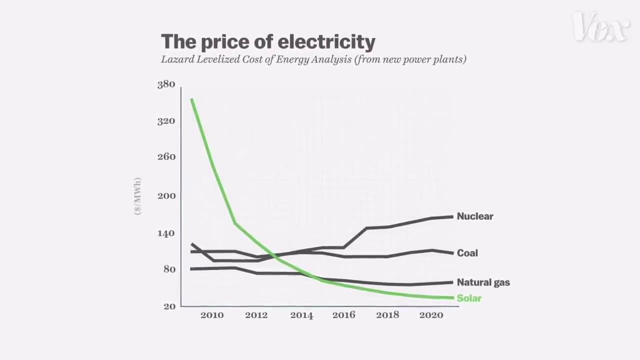 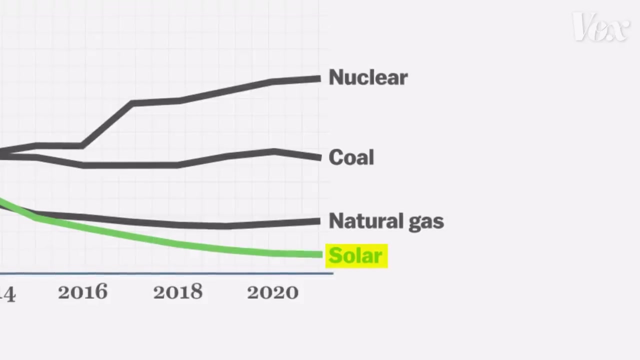 the biggest producer of solar, but the biggest producer of solar electricity. In the course of a single lifetime, solar energy has transformed from a niche technology to the cheapest way to bring clean, reliable power to billions of people around the world. But the markets that brought us these lower prices didn't just magically appear by some. 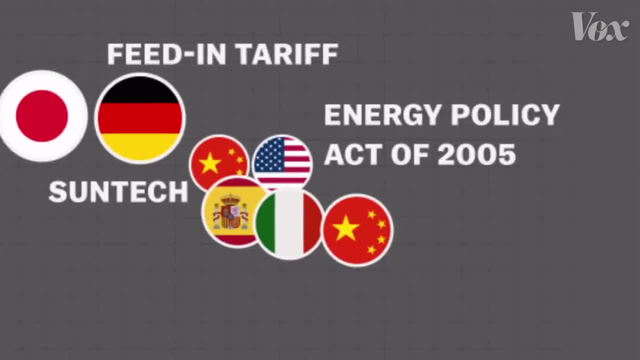 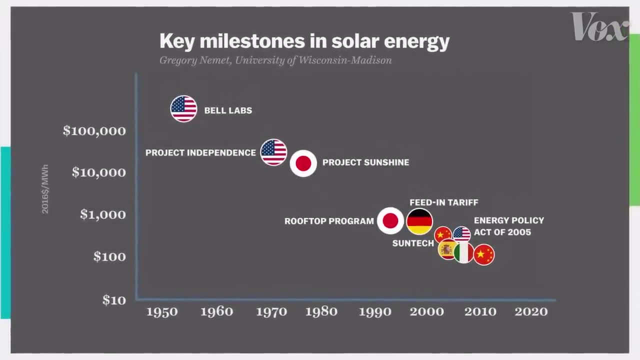 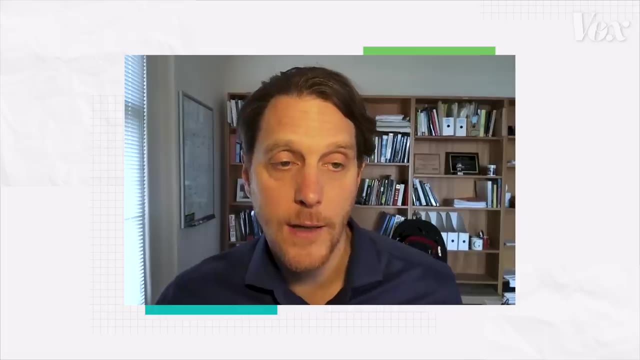 invisible hand. Political leaders in countries all over the world created these markets, then subsidized them for decades to the tune of billions of dollars. By investing that money, you got the solar to come down in costs to the point where you don't need to subsidize it anymore. We're doing that on purpose with